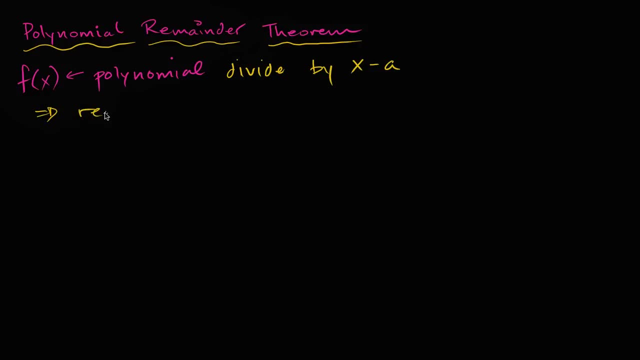 then the remainder, then the remainder from that essentially polynomial long division is going to be f of a. It is going to be. it is going to be f of a, f of a. I know this might seem a little bit abstract, but right now I'm talking about f of x's and x minus a's. 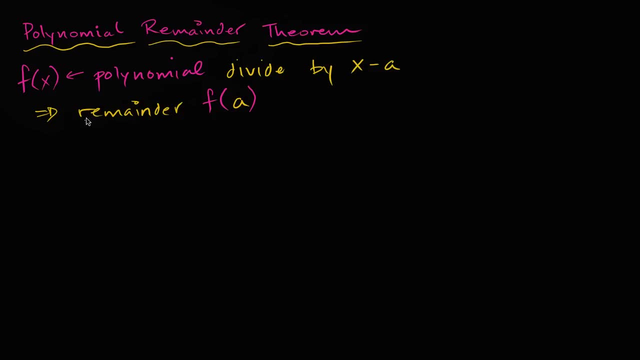 Let's make it a little bit more concrete. So let's say that f of x, f of x is equal to. I'm just going to make up a, let's say, a second degree polynomial. This would be true for any polynomial, though. 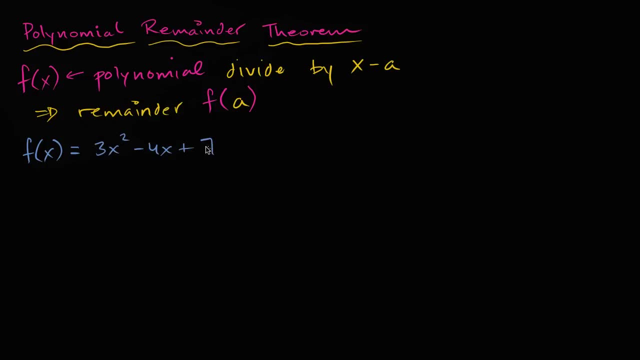 So three x squared minus four, x plus seven, And let's say that a is- I don't know- a is one. So we're going to divide by, we're going to divide that, we're going to divide by x minus x minus one. 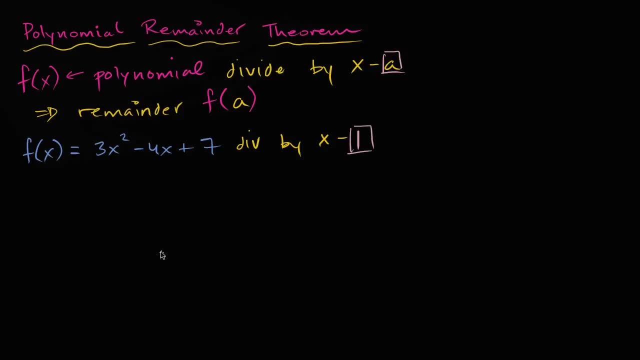 So a in this case is equal to one. So let's just do the polynomial long division, and I encourage you to pause the video. and if you're not unfamiliar with polynomial long division, I encourage you to watch that before watching this video, because I will assume you know how to do. 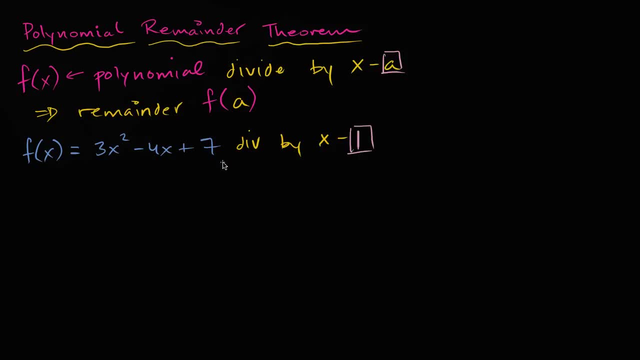 polynomial long division. So divide three x squared minus four, x plus seven. Divide it by x minus one, See what you get as your remainder and see if that remainder really is f of one, Assuming you've had a go at it, so let's work through it together. 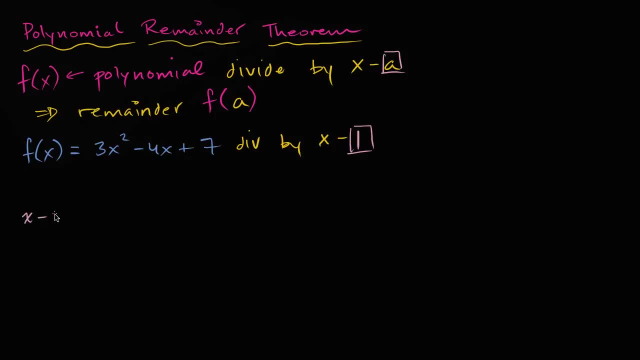 So let's divide x minus one, x minus one into three, x squared into three, x squared minus four, x plus seven. All right, a little bit of polynomial long division is never a bad way to start your morning. It's morning for me. 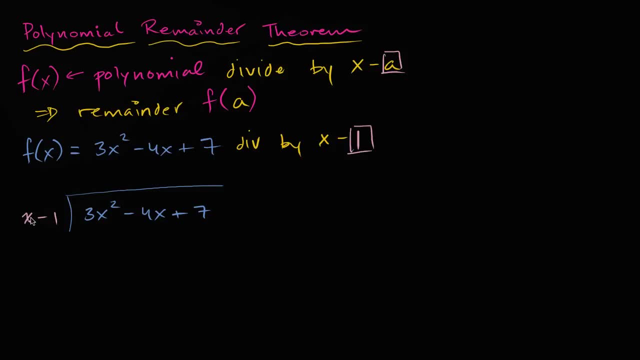 It is for you All right. so I always look at the x term here, the highest degree term, and then I'll start with the highest degree term here. So how many times does x go into three x squared? Well, it goes three x times. 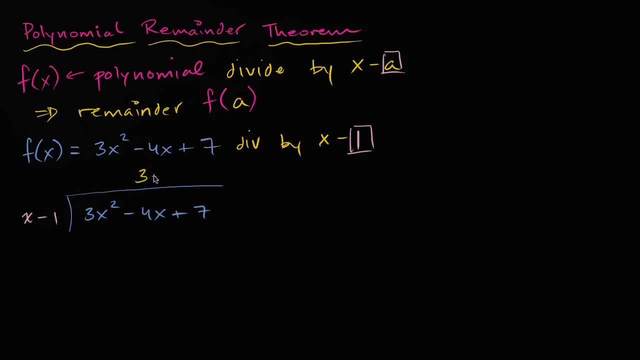 Three x times x is three x squared. so I'll write three x over here. I'm writing it in the- I guess you could say the first degree place. Three x times x is three x squared. Three x times negative one is negative three x. 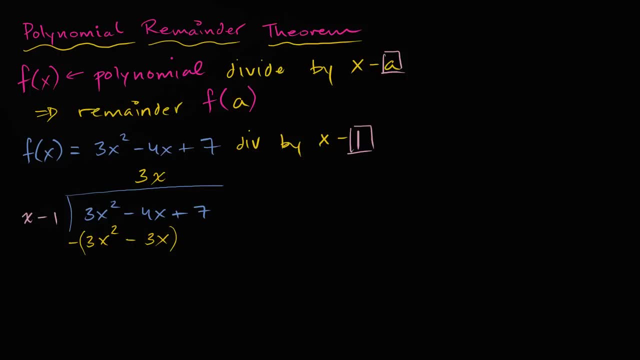 and now we want to subtract. we want to subtract this thing. This is just the way that you do traditional long division. And so what do we get? Well, three x squared minus three x squared, that's just going to be zero. 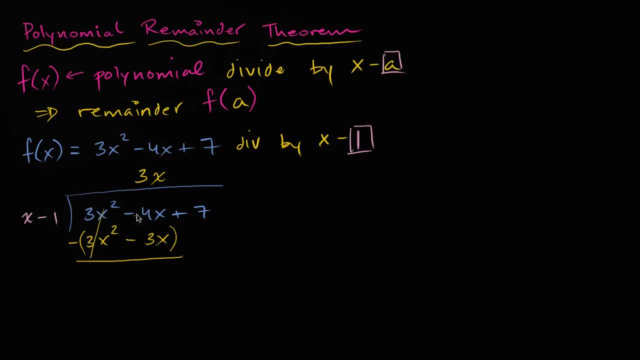 So these just add up to zero And this negative four x, this is going to be plus three x. right, A negative of a negative. Negative four x plus three x is going to be is going to be negative x. Let me do this in a new color. 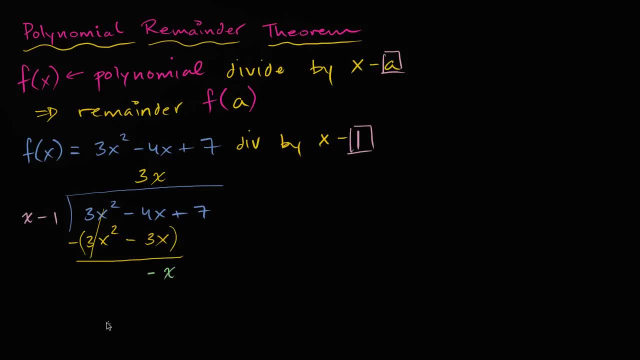 So it's going to be negative, negative x, and then we can bring down. we can bring down the seven. Complete analogy to how you first learn long division in maybe- I don't know- third or fourth grade. So all I did is I multiplied three x times this. 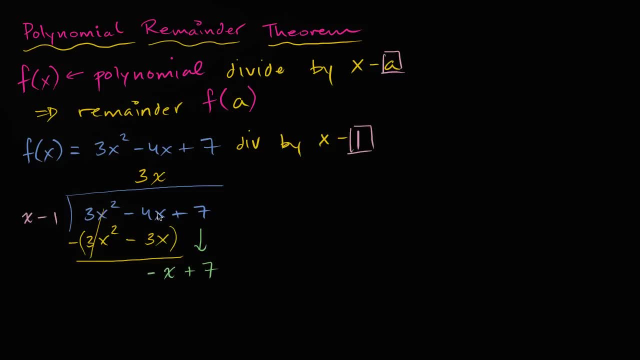 You get three x squared minus three x, and then I subtracted that from three x squared minus four x to get this right over here. Or you could say: I subtracted it from this whole, from the whole polynomial, and then I got negative x plus seven. 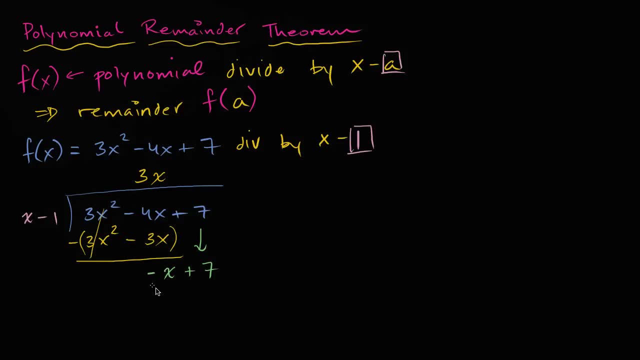 So now, how many times does x minus one go into negative, x plus seven? Well, x goes into negative, x negative, one times Negative, one times Negative. one times x is negative, x Negative, one times negative, one is positive one. But then we're going to want to subtract this thing. 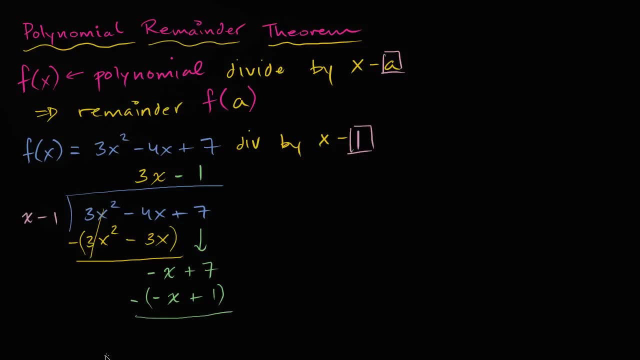 We're going to want to subtract this thing and this is going to give us our remainder. So negative x minus negative x, that's the same thing as negative x plus x. So that's, these are just going to add up to zero. 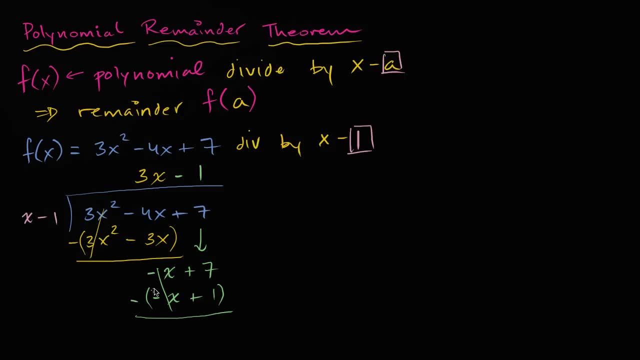 And then you have seven. This isn't going to be seven plus one. Remember, we have this negative out. So if you distribute the negative, this is going to be a negative one. Seven minus one is six, So your remainder here is six. 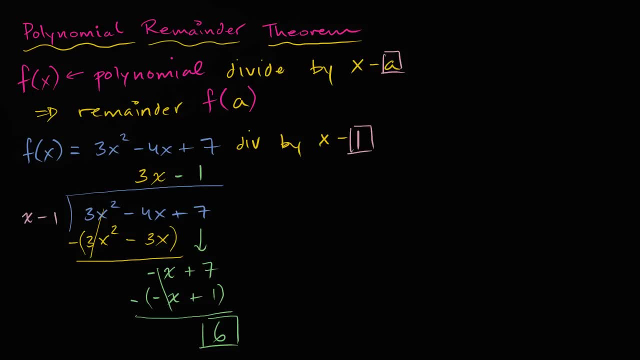 One way to think about it. you could say. you could say that you could say: well, actually, I'll save that for a future video. This right over here is the remainder, Remainder, And you know when you got to the remainder. 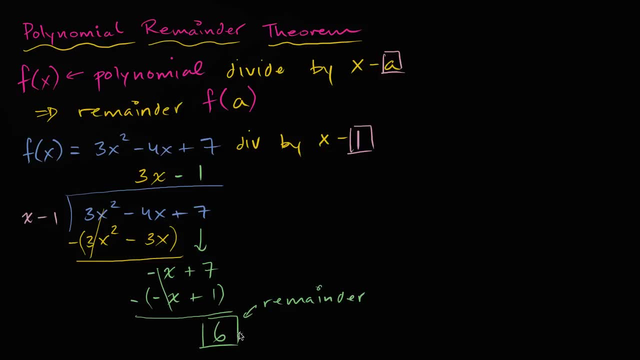 and this is just all a review of polynomial. long division is when you get something that has a lower degree. This is a- I guess you could call this a- zero degree polynomial. This has a lower degree than what you are actually dividing into.